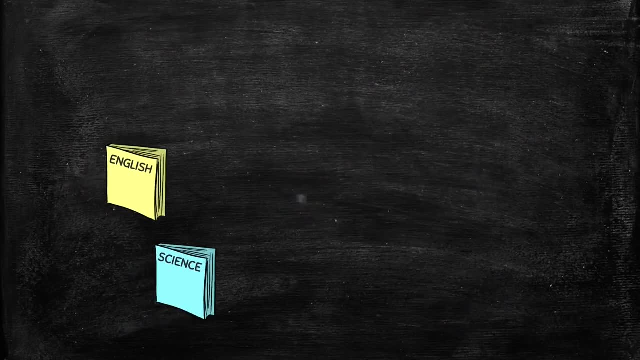 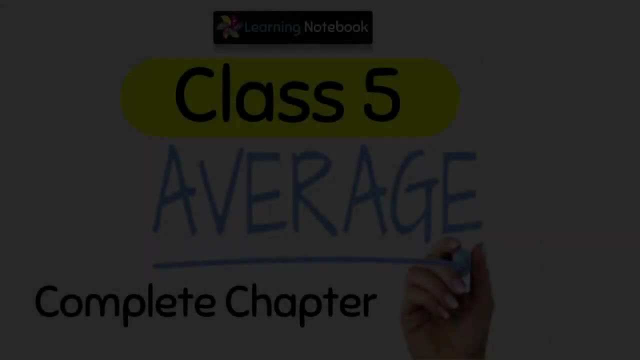 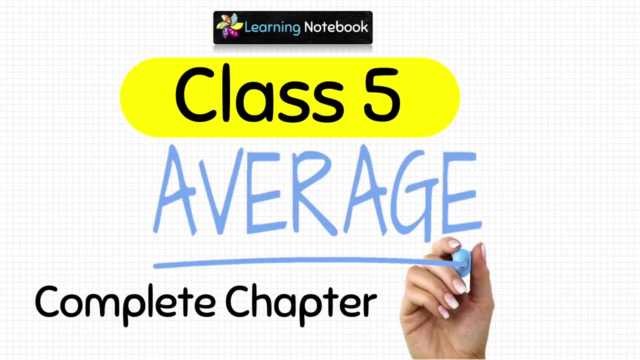 Hello students, welcome to our channel Learning Notebook. In today's video we are going to do complete chapter of average for class 5.. In this video we are going to discuss each and every concept related to average, So make sure you watch the entire video. 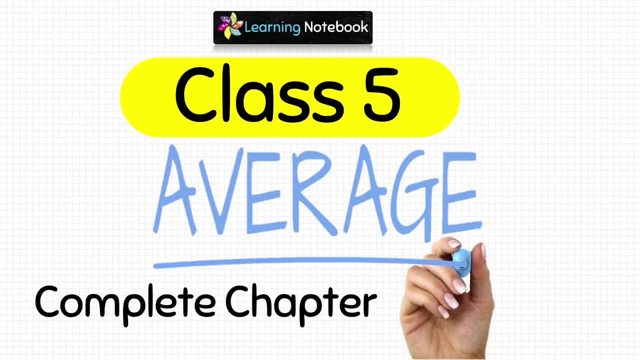 But before starting with this chapter, let me tell you that we have made videos on every chapter of class 5, mathematics. We also have interesting worksheets and quizzes on each chapter. You can find all of them on our channel, Learning Notebook. Also, you can see a list of all such videos on our website. 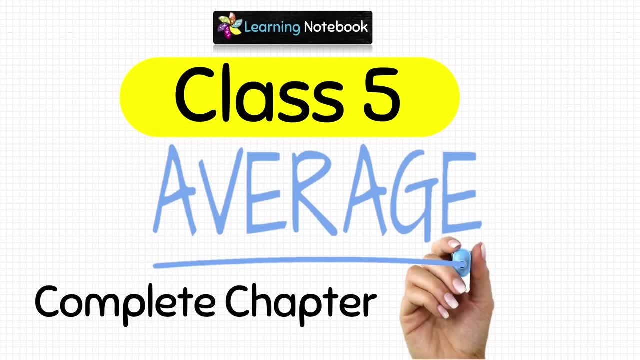 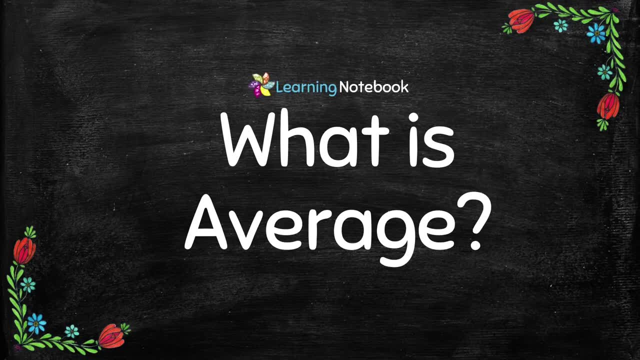 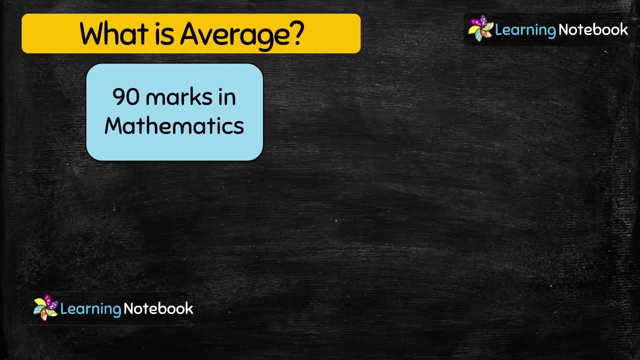 The link to our website is below in the description box. So let's start with this chapter and first understand what is the meaning of average. To understand this concept, let's take an example. Suppose a student has secured 90 marks in mathematics. 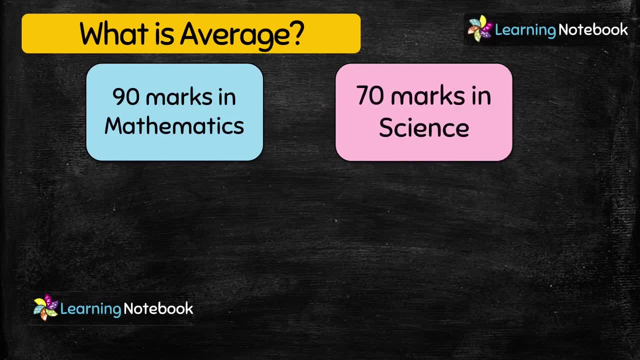 And 70 marks in science. Now he wants to know his average score per subject. So here we need to find average. How many subjects do we have here? Two, So to find average we will just add the marks of both these subjects. 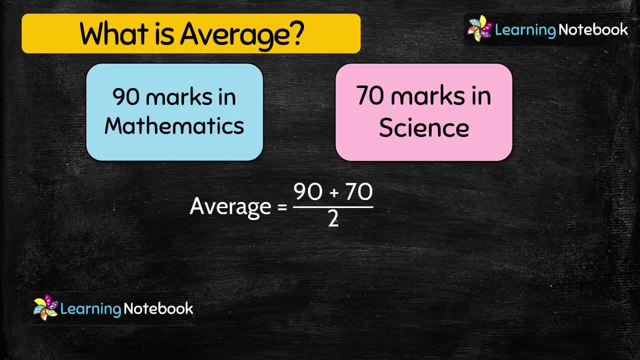 And divide it by 2.. So we will do 90 plus 70 divided by 2.. 90 plus 70 equal to 160. And 160 divided by 2 equal to 80. So we have got the average as 80 marks per subject. 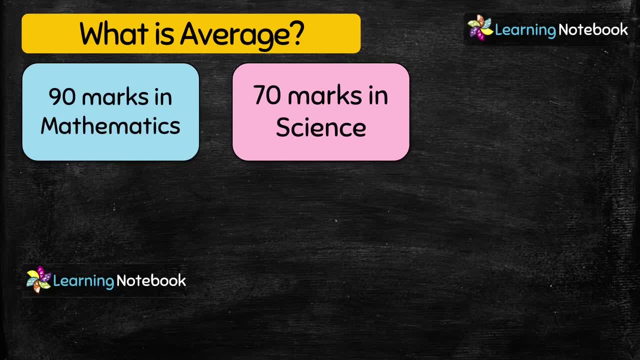 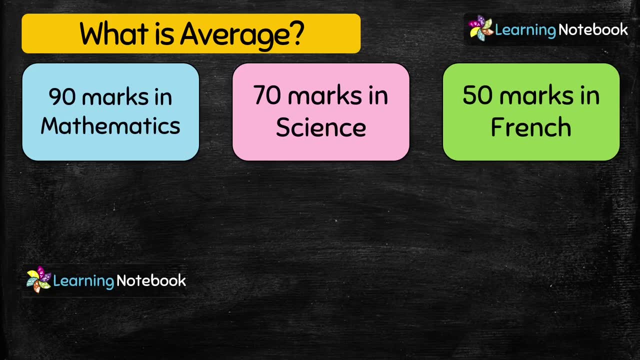 So this means the average is 90. And we will add more marks for each subject. Now he has got the result of his third subject, which is French, And he has secured 50 marks in French, And again he wants to know his average per subject. 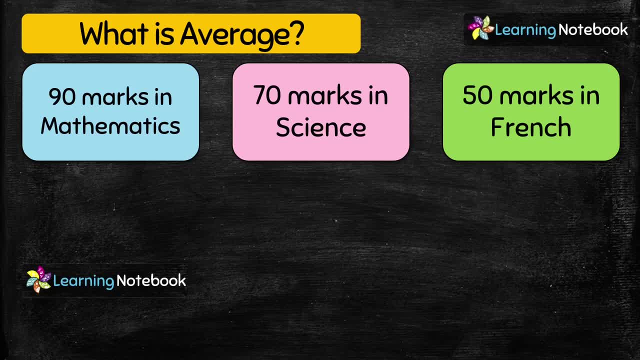 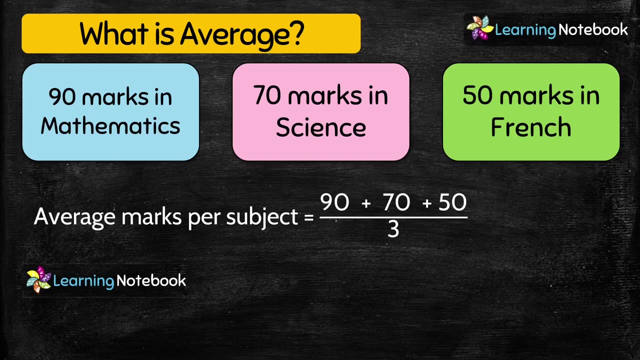 So this time again we are going to add the marks of all the 3 subjects. So this time again, we are going to add the marks of all the 3 subjects, subjects, and we will divide it by 3, because number of subjects have increased to 3.. 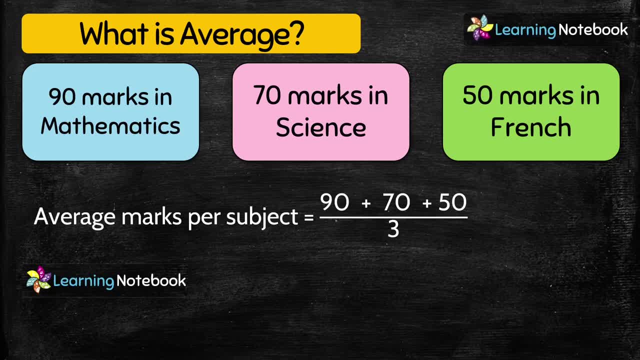 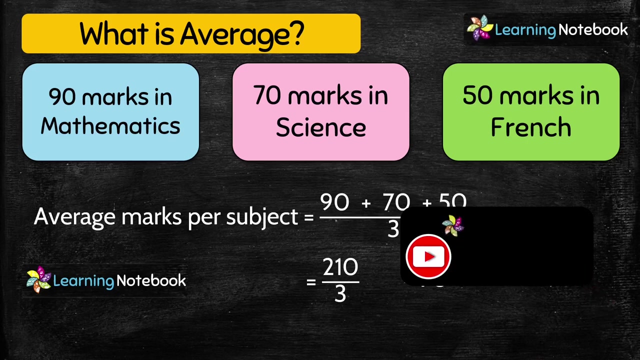 So we will do 90 plus 70 plus 50 divided by 3.. After adding the marks, we have got 210 divided by 3, which is equal to 70.. So, students, did you notice that average marks per subject have now changed to 70.? 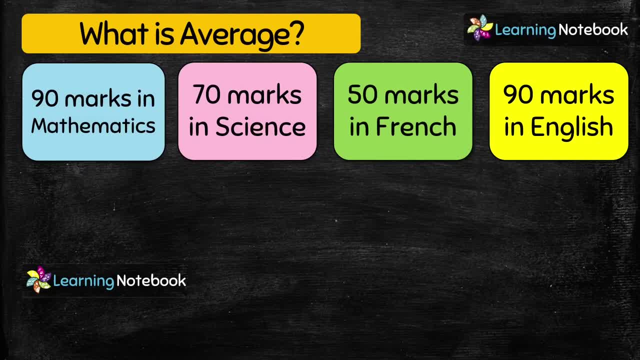 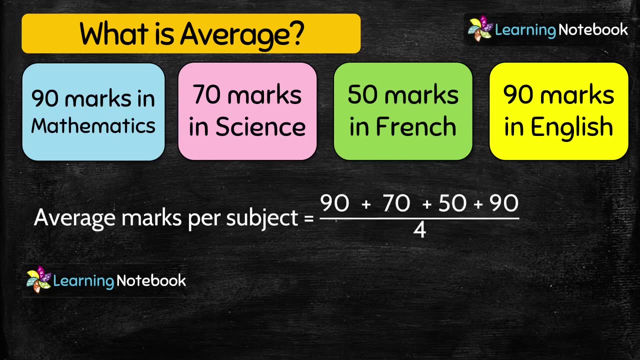 Next, let's suppose he has also got the marks for English subject. So now what will he do To calculate the average marks? yes, this time we will divide the sum of all the subjects by 4.. So we will do 90 plus 70 plus 50 plus 90 divided by 4, and we get the sum as 300 and we will divide it by 4.. 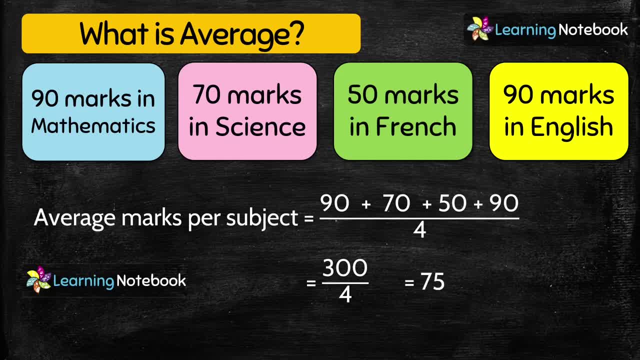 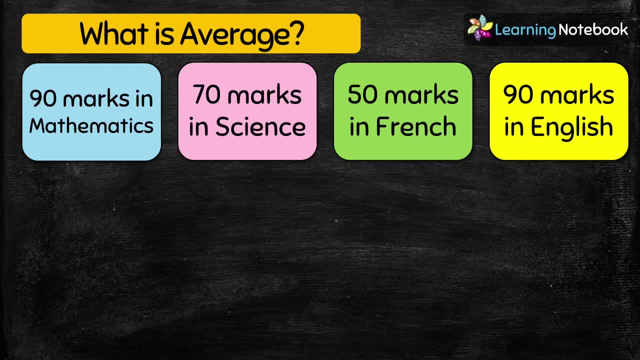 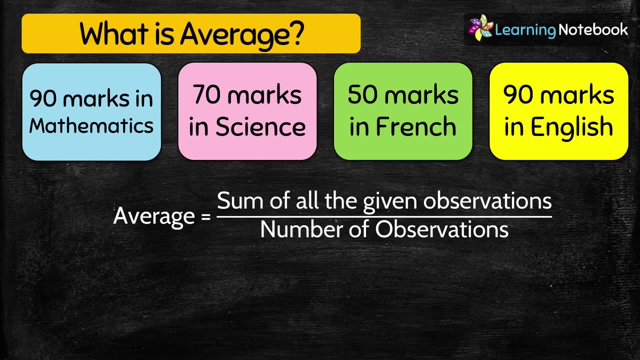 And we get the sum as 300 and we will divide it by 4.. And we get the sum as 300 and we will divide it by 4.. So we now calculate the average marks per subject as 75. So, students, in general we can say average equal to sum of all the given observations divided by number of observations. 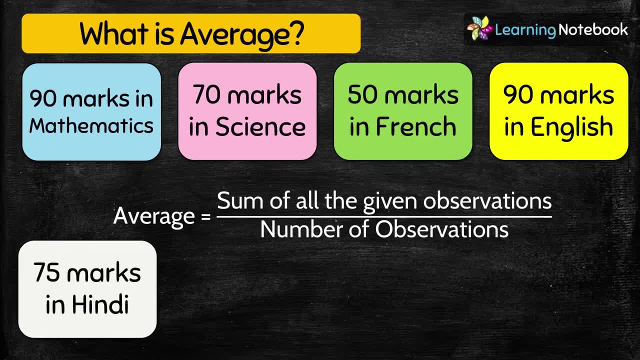 So students in general, we can say average is 75. Now, luminance region less than zero is моя foundation. So, students in general, thousand is my foundation, So here you should be able to use your Tisch. So, students in general, thousand is my foundation. 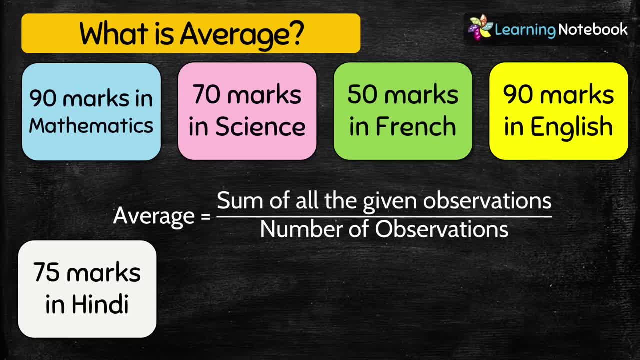 So, students in general, we can use your Tisch for Hindi as well, and he has secured 75 marks in Hindi. so, students, now I would like you to calculate the average marks per subject and do write your answer in the comment section below, just to give you a little hint. this time we will. 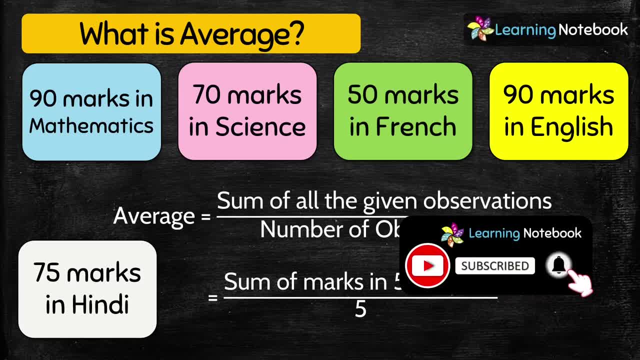 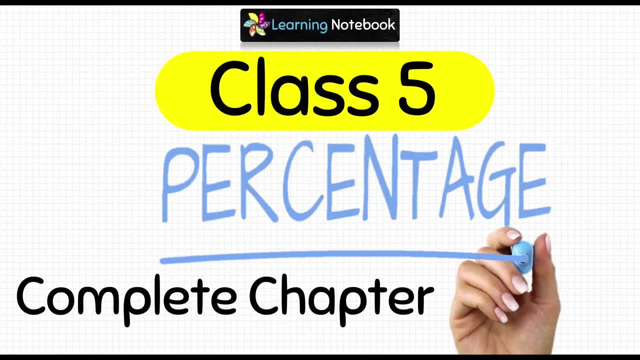 divide by 5, as there are five subjects. we also have a separate video on complete chapter of percentage for class 5. I'm sure all your doubts related to this concept would be resolved after watching this comprehensive video. you will find its link here on the top and. 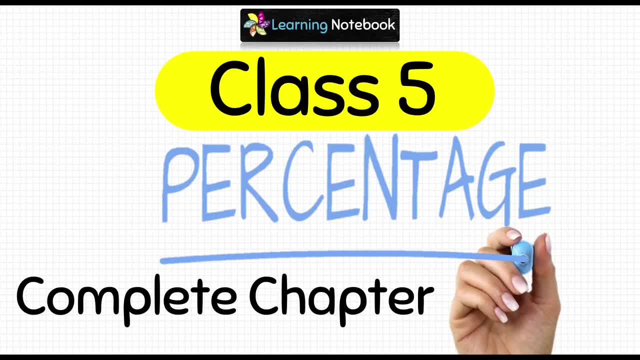 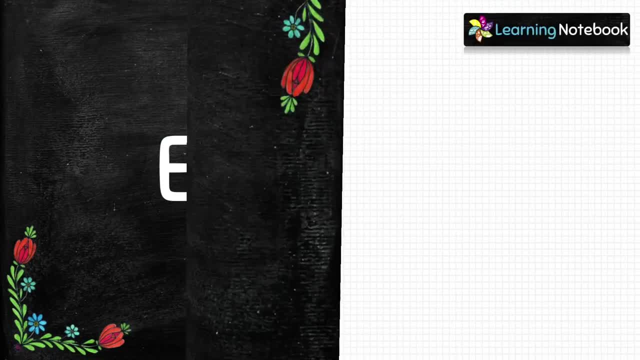 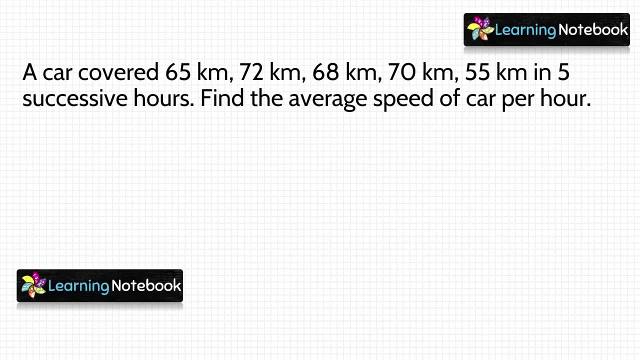 below in the description, below description box. Lets do some exercise Now. lets do some exercise. question 1.A car covered: 65km, 72 km, 68 km, 70 km, 55 km in 5 successive laps, 85 km in 5 successive laps. 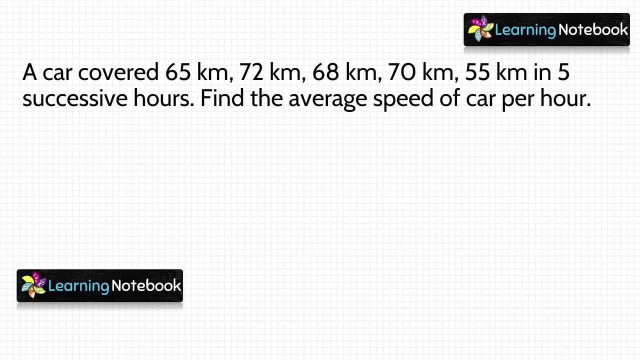 груп in 2 times 65 km, 70 km, 65 km in 5 successive laps- false successive hours- find the average speed of car per hour. so here, students, we have to find the average speed of the car per hour, and we know speed equals to distance covered upon. 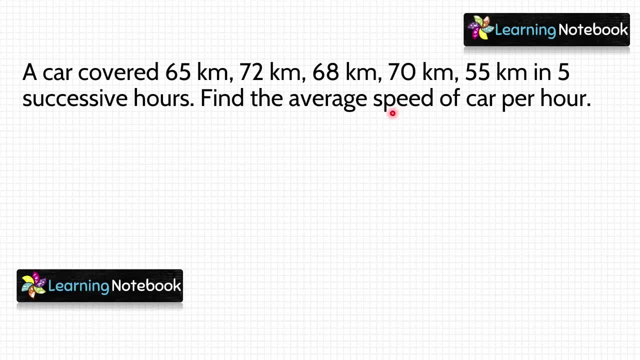 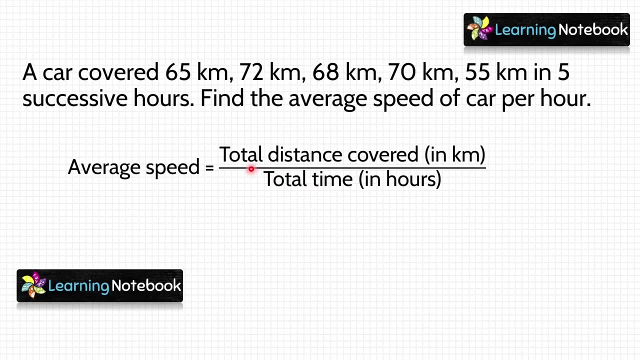 time taken. so average speed will be total distance covered divided by total time taken, and total distance covered will be sum of all these distances, and total time taken is 5 times total distance covered. So let's write it as 65 plus 72 plus 68 plus 70 plus 55 divided by 5. now let's add them. 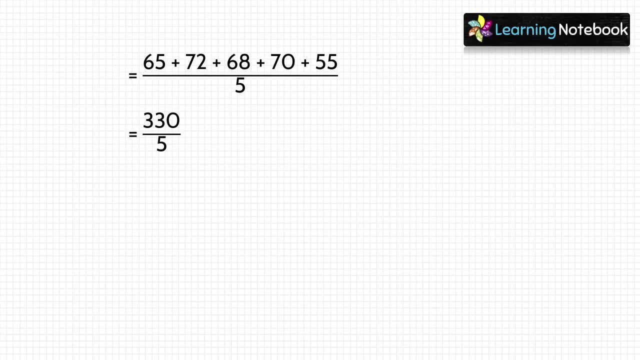 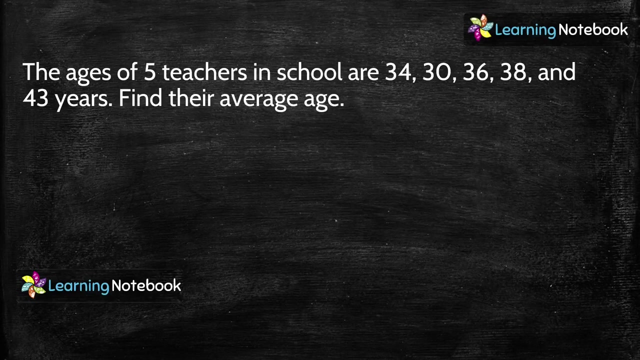 and we get the sum as 330 divided by 5 and we get the average speed of the car per hour and we get the answer as 66. so average speed of car is 66 kilometer per hour. let's see the next question. the ages of five teachers in a school are 34, 30, 36, 38 and. 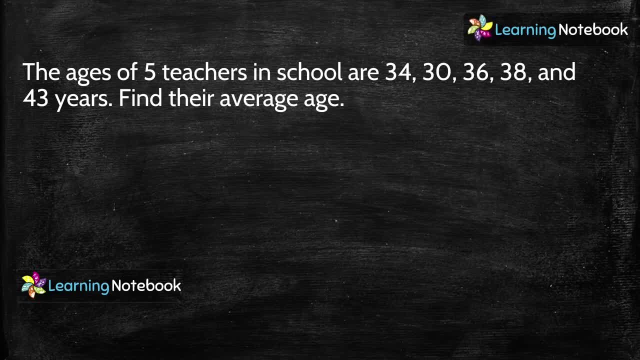 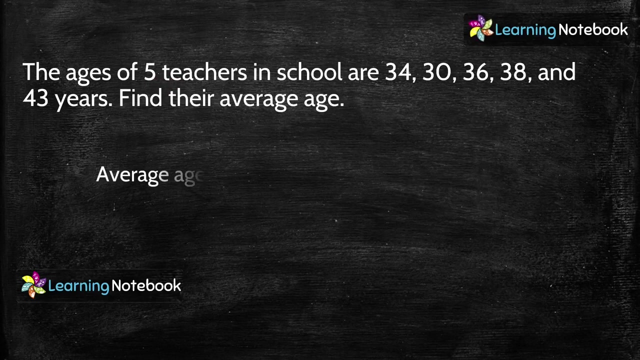 43 years, find their average age. so here we are, given the age of five teachers and we have to find their average age. so first we will add all these five ages and we will divide that sum by number of teachers, which is five. so let's solve it. average age equal to sum of ages of 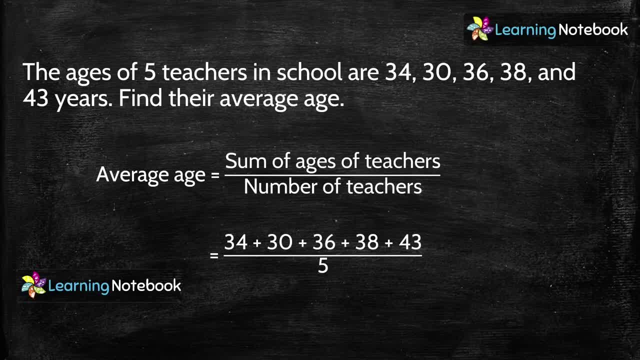 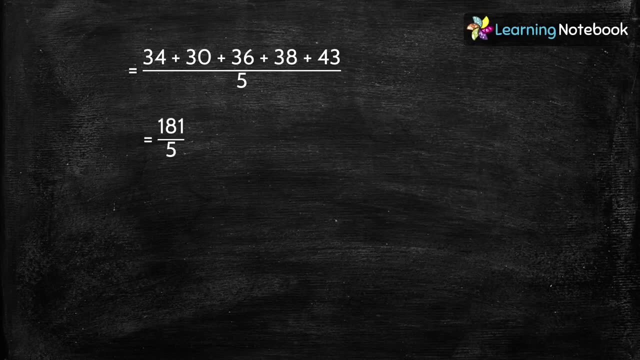 teachers, divided by number of teachers. so let's add all these five ages and divide it by five. now, by adding these five numbers, we get the sum as 181: 1. Let's divide it by entitles. divide it by 5. Now, students, as you can see, the remainder is one, so we can still. 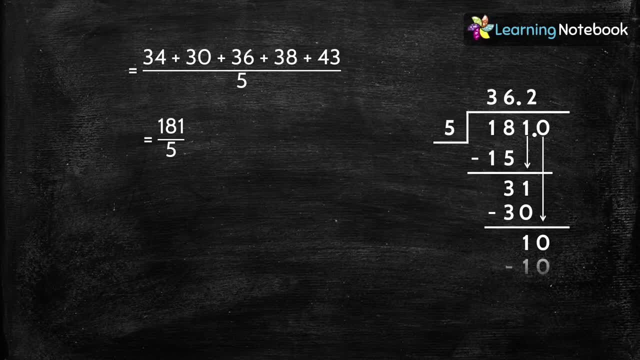 Right now is 181. now, students, as you can see, the reminder is one, so we can still continue. right now is 181. now, students, as you can see, the remainder is one, so we can still繼續 with the division by inserting a decimal point and a zero. so we have got the. 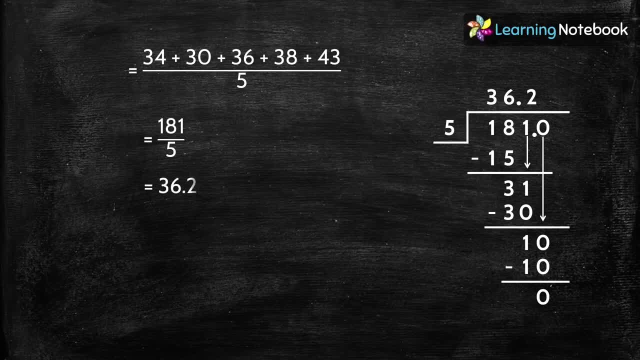 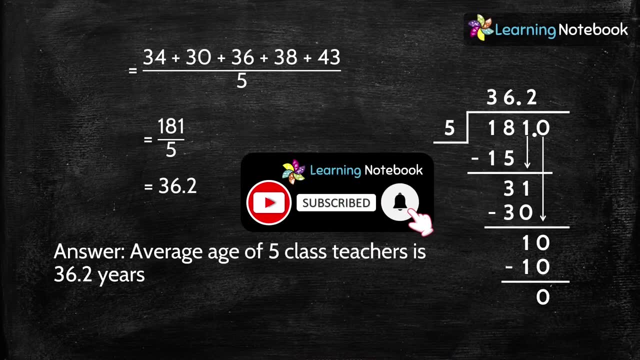 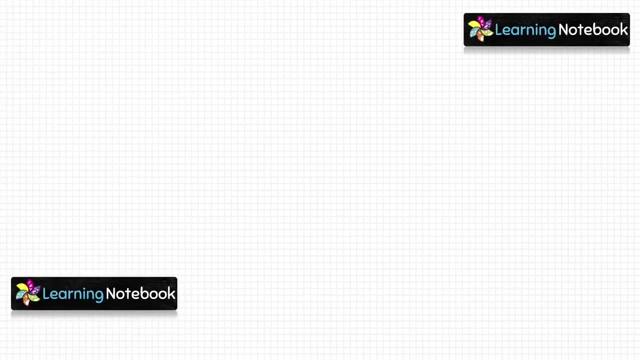 quotient as 36.2. so answer is: average age of five class teachers is 36.2 years. let's move to next question: find the average of all odd numbers between 20 and 40. so let's first understand this question here. first we need to find the 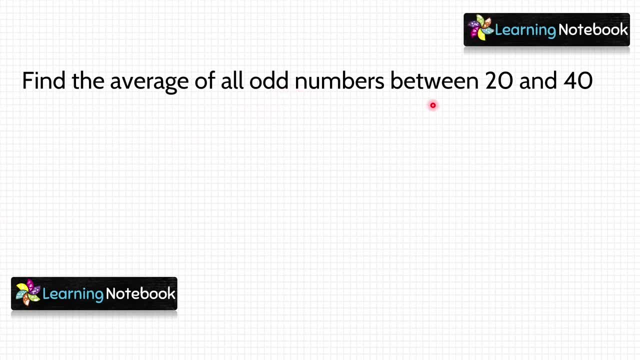 odd numbers between 20 and 40 and then we will add all those numbers and divided by number of odd numbers. so let's see how to solve it. so let's first write the odd numbers. so odd numbers between 20 and 30 are 21,, 23,, 25,, 27,. 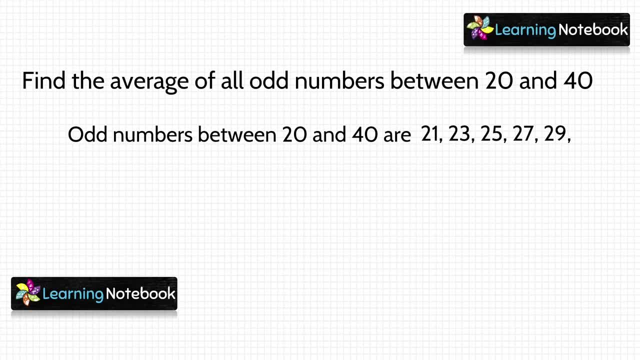 and 29.. And odd numbers between 30 and 40 are 31,, 33,, 35,, 37 and 39.. So these are all the odd numbers between 20 and 40.. How many are these? Count them: These are 10 odd numbers. So now, 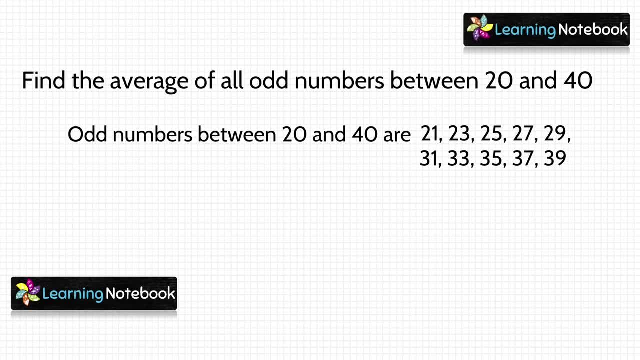 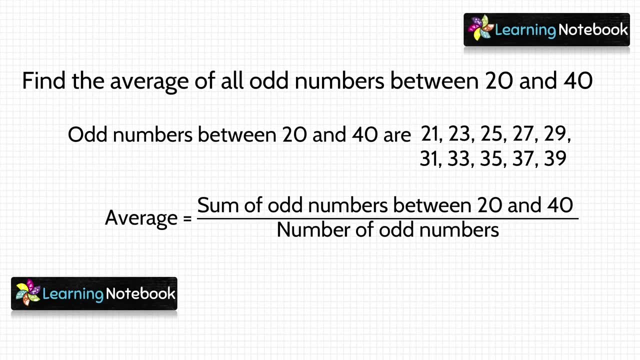 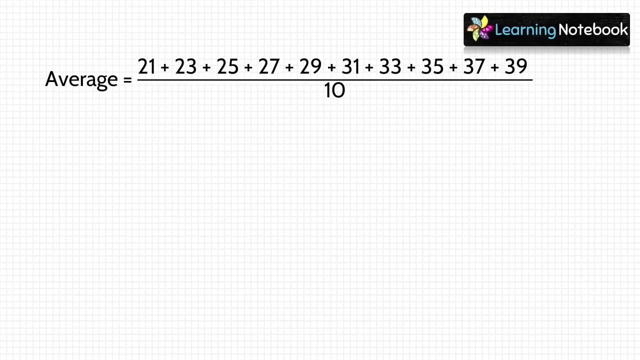 we have got all the information, So let's find the average. We will add all these 10 odd numbers and divide that sum by number of odd numbers, which is 10.. Now, by adding these 10 numbers, we get the sum as 300.. 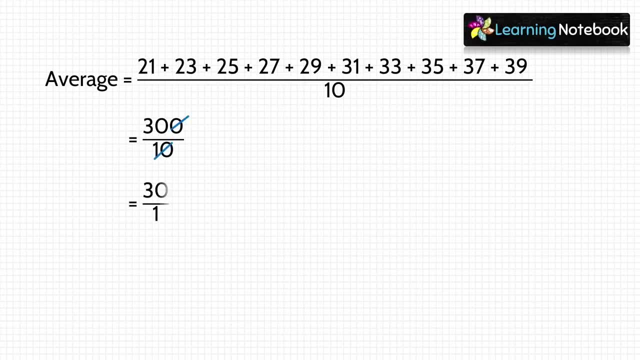 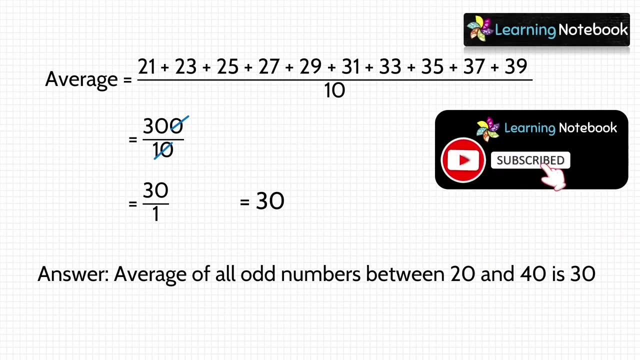 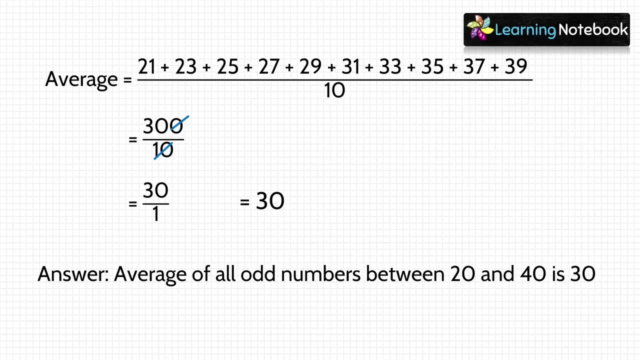 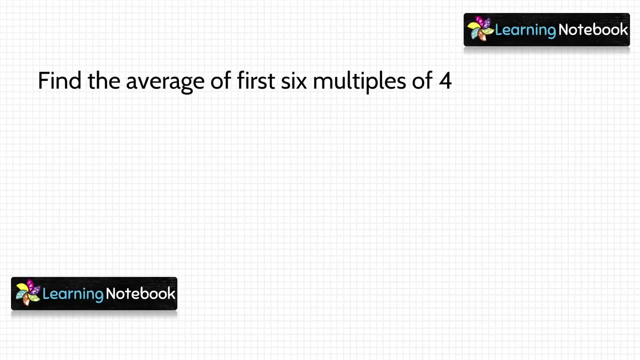 Let's divide it by 10. Cancel 0 by 0 and we get the answer as 30. So average of all odd numbers between 20 and 40 is 30.. Let's do another question: Find the average of first 6 modules. 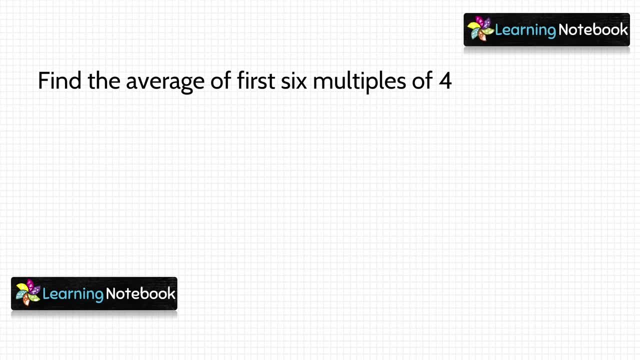 So here, students, first we need to find the first 6 multiples of 4 and then we will add them and divide them by total number of multiples. So first 6 multiples of 4 are 4,, 8,, 12,, 16,. 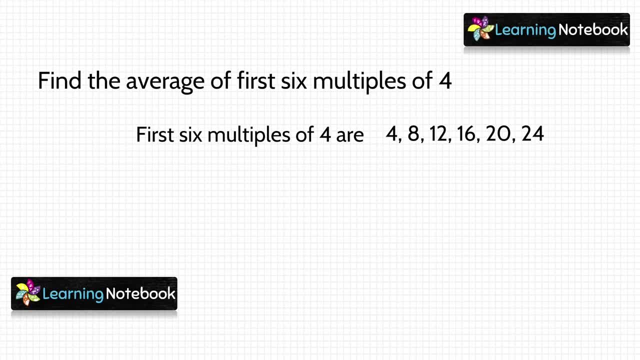 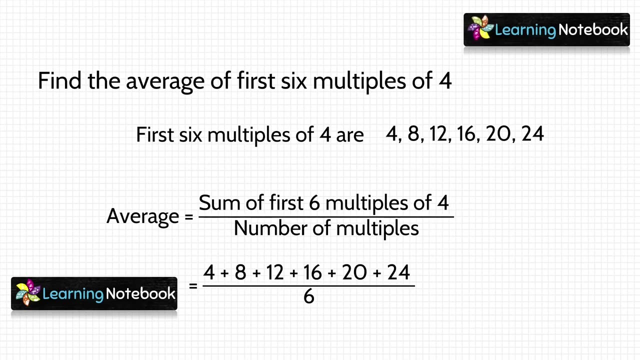 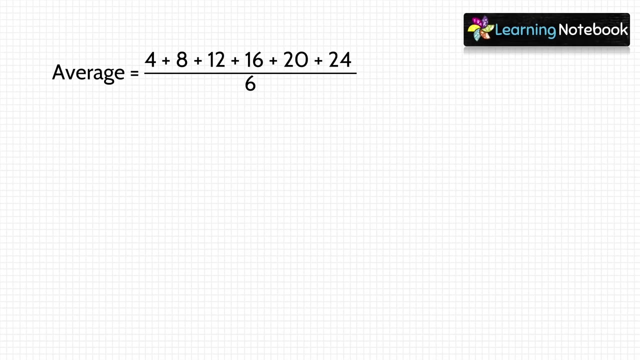 20 and 24.. Now, to find their average, let's add all these 6 multiples and divide the sum by number of multiples, which is 6.. By adding these 6 numbers, we get the sum as 85. So we have got the sum as 85.. So now let's find the average of all odd numbers. So here, students, first 6 numbers, we get the sum as 85.. So here, students, first 6 numbers, we get the sum as 85.. So here, students, first 6 numbers, we get the sum as 85.. 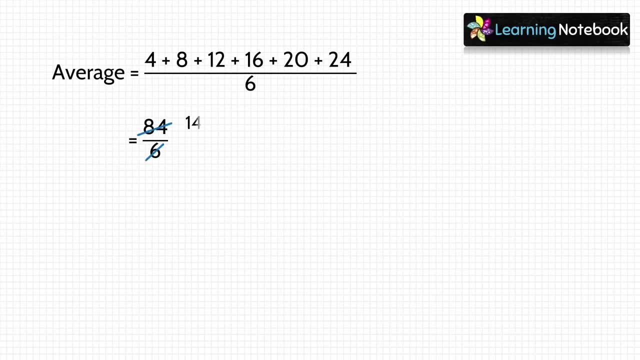 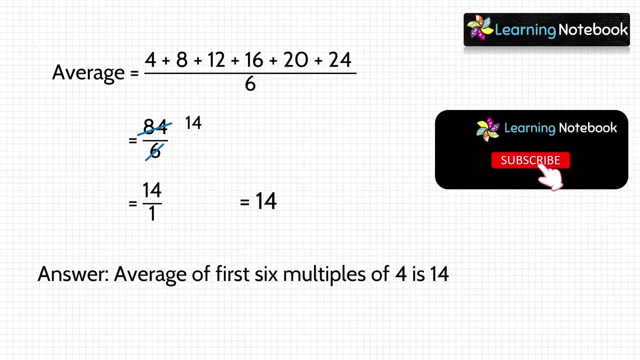 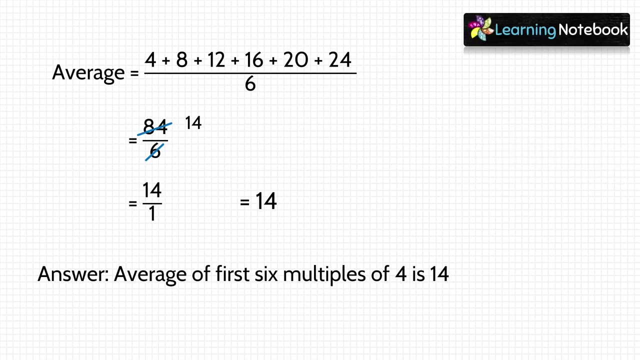 Let's divide 84 by 6 and we get the answer as 14.. So average of first 6 multiples of 4 is 14.. If you still not have subscribed to our channel Learning Notebook, then do subscribe it And make sure to press the bell icon. 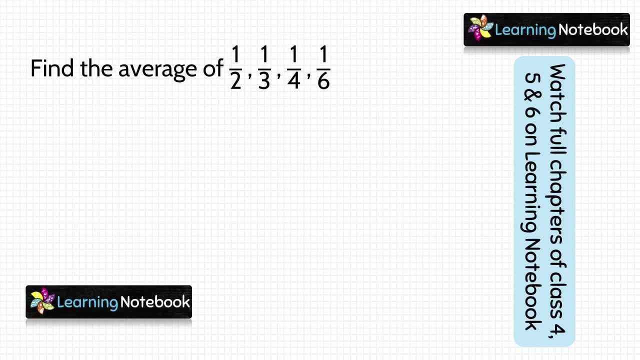 Let's do a different question now: Find the average of 1 by 2,, 1 by 3,, 1 by 4 and 1 by 6.. So here, students, we have to find the average of 4 fractions. 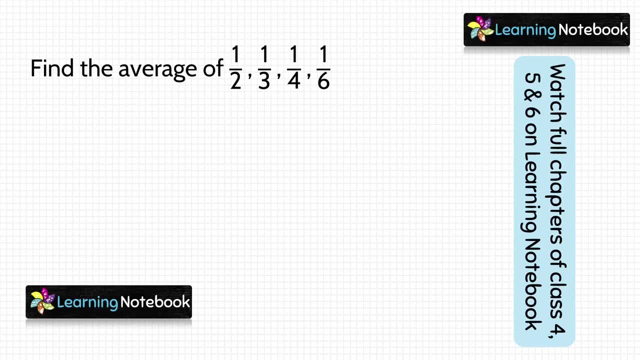 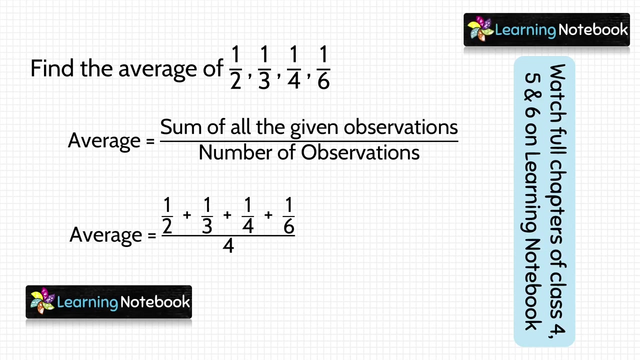 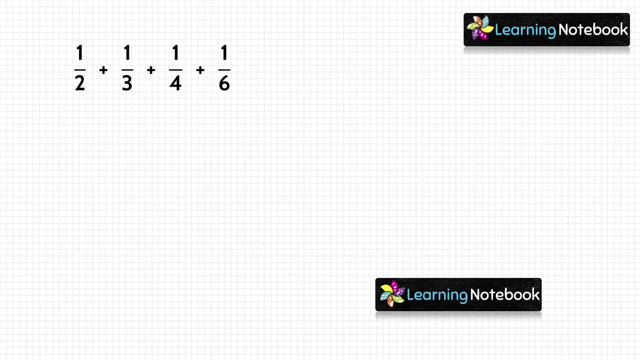 So let's solve it First. we know average equal to sum of all the given observations divided by number of observations. So we will first add all these 4 fractions and then divide that sum by 4, which is number of fractions. So let's first add 4 fractions. 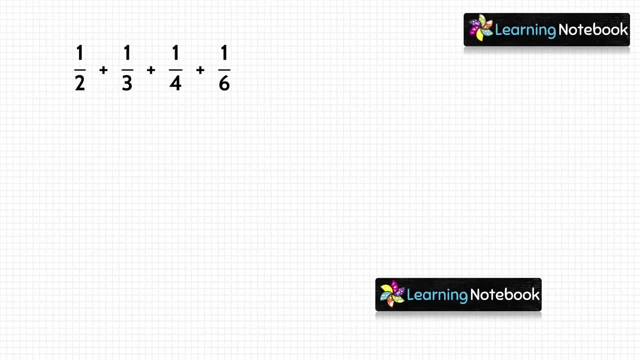 And then we will add these fractions. But, students, these are unlike fractions, So first we will have to find their LCM to convert them into like fractions. So we will find the LCM of their denominators 2, 3,, 4 and 6.. 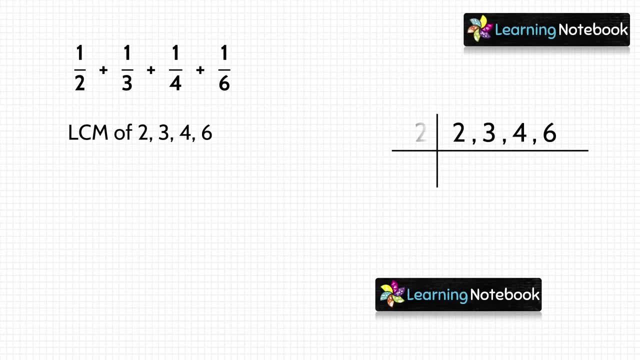 Let's first divide them by 2.. Then we will divide them by 3. And finally we will divide them by 2.. So LCM of their denominators is 2 multiplied by 3, multiplied by 2, which is equal to 12.. 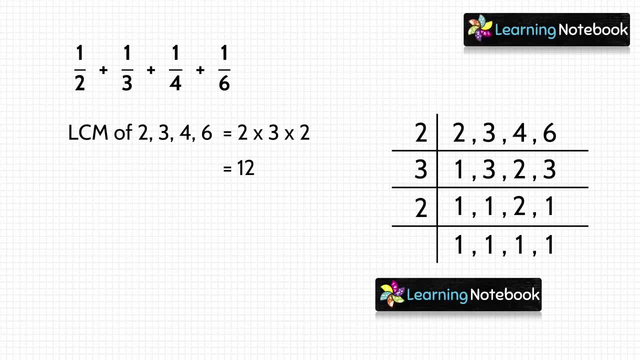 Now we will convert these unlike fractions into like fractions By converting their denominator equal to 12.. So first let's convert 1 by 2 into equivalent fraction of denominator 12.. So we will multiply both numerator and denominator by 6.. 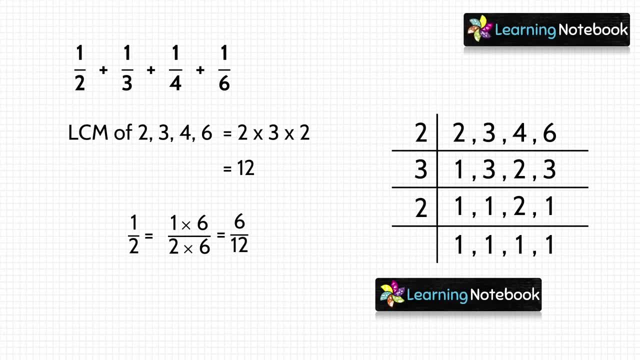 We get 6 by 12.. Similarly, let's convert, Let's convert second fraction, 1 by 3, into equivalent fraction of denominator 12.. So we will multiply both numerator and denominator by 4.. We get 4 by 12.. 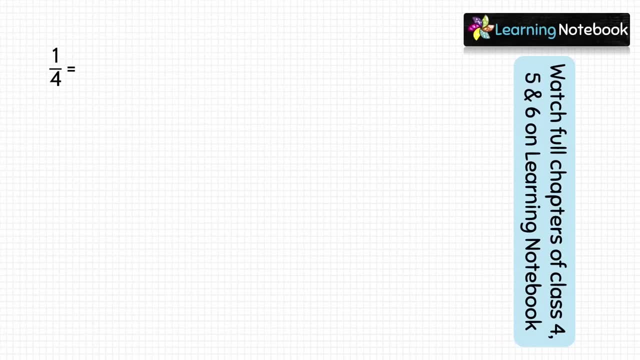 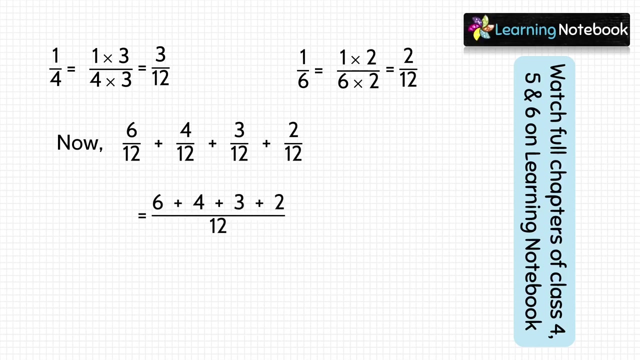 In the same way, let's convert the remaining 2 fractions into equivalent fractions of denominator 12.. So we did that. So now, students, we have converted all the fractions into like fractions And we can easily add them now. So let's just add their numerators. 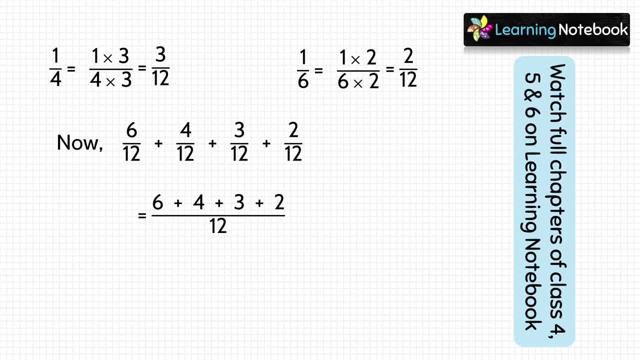 And denominator remains the same as 12. So 6 plus 4 plus 3 plus 2 equal to 15. So we get the sum as 15 by 12. Let's simplify it by dividing with common factor 3 And we get 5 by 4. 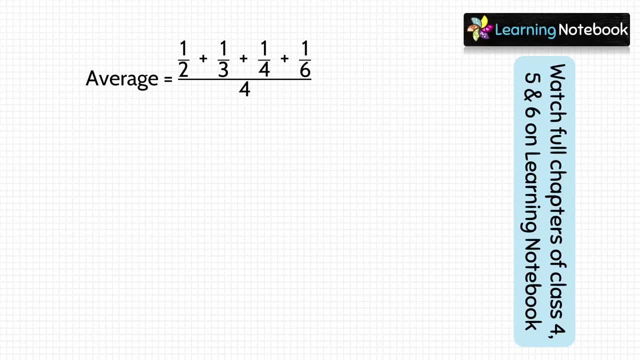 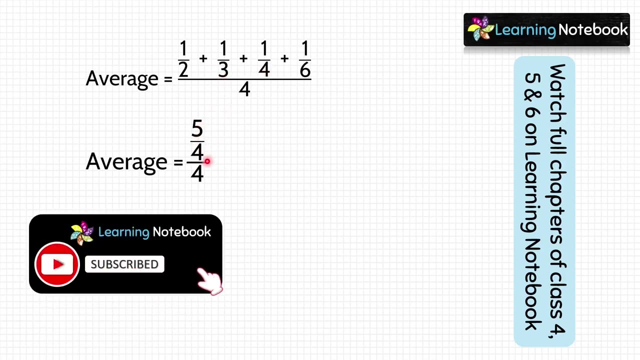 Now, students, we know the sum of all these fractions, So let's find the average Average equal to 5 by 4, divided by number of fractions, which is 4. For those of you who do not know how to solve this type of division, Think this fraction 5 by 4 standing on a chair. 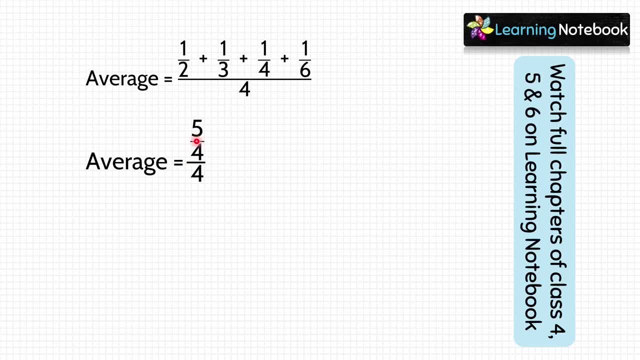 Now 5 by 4 cannot keep on standing, So when 5 by 4 will sit on the chair, This 4 will become its denominator. So we get 5 divided by 4 into 4, Which is equal to 5 by 16. So average of these 4 fractions: 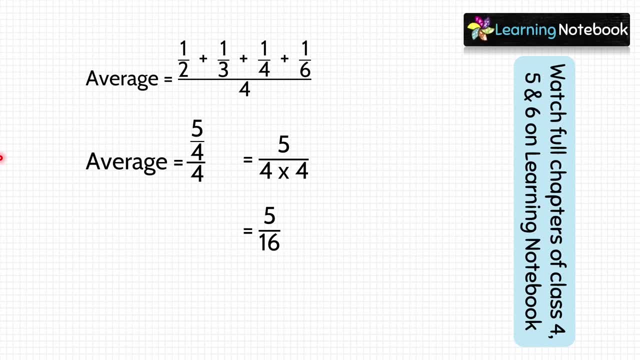 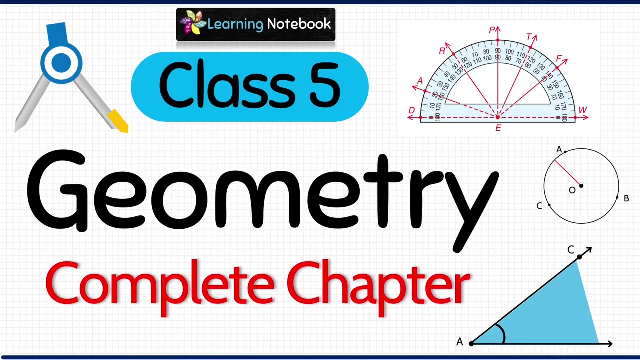 Is 5 by 16. Students do practice such type of questions As these are important from exam point of view. We also have a separate video On complete chapter of geometry for class 5. I am sure all your doubts related to this chapter Will be answered in the next chapter.